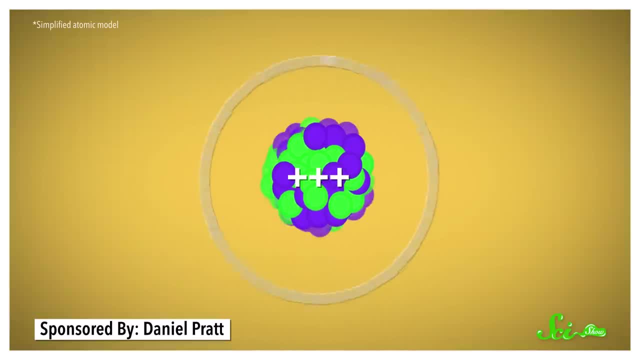 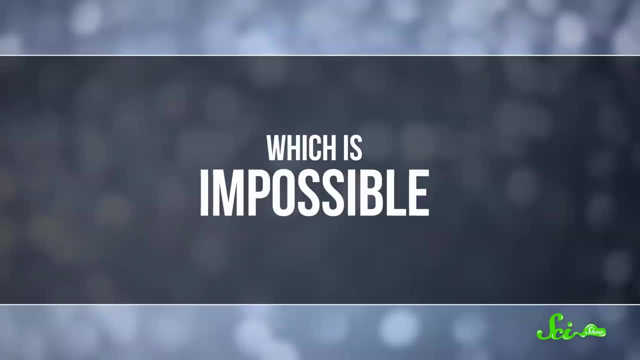 So the electrons have to go faster, and faster the bigger the nucleus gets. Feynman showed that in an atom with 137 protons, electrons would be moving faster than the speed of light. And going faster than the speed of light is impossible. 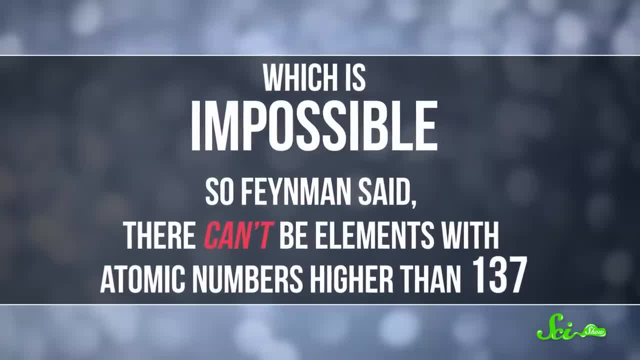 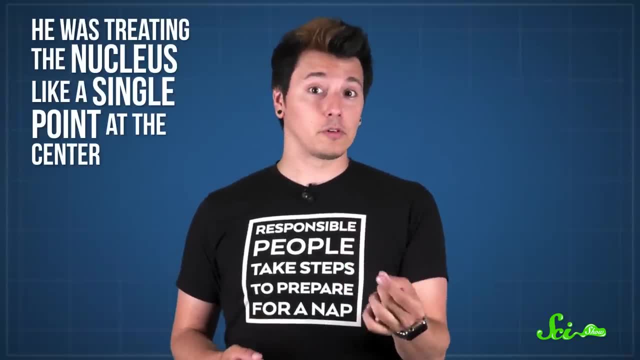 So Feynman said there can't be elements with atomic numbers higher than 137. He might have been wrong, though His calculations made sense. but he was treating the nucleus like a single point at the center of the atom. That works fine for smaller nuclei, but it doesn't work very well for the hulking masses we're talking about here. 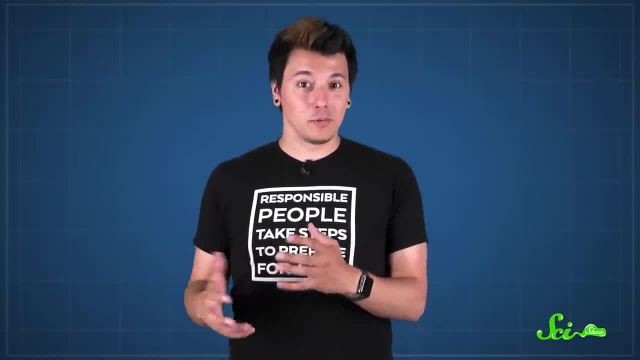 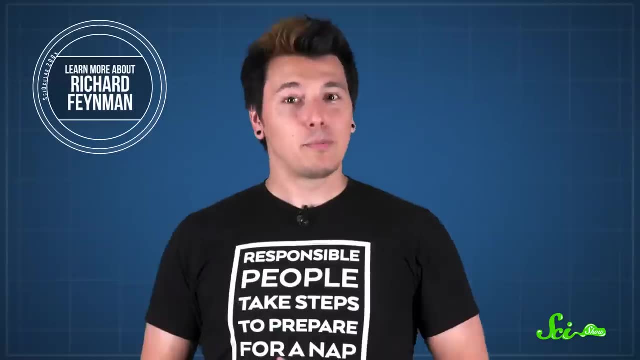 Physicists and chemists have even joked that element 137,, once it's finally created, should be named Feynminium, Respectfully making fun of the Nobel Prize winning physicist. for one of the few things he was wrong about, He probably would have liked that. When Feynman's calculation is repeated in a way that does account for the size of the nucleus, the number gets pushed all the way up to 173.. In atoms with more than 173 protons, electrons really do seem to need to go faster than the speed of light. 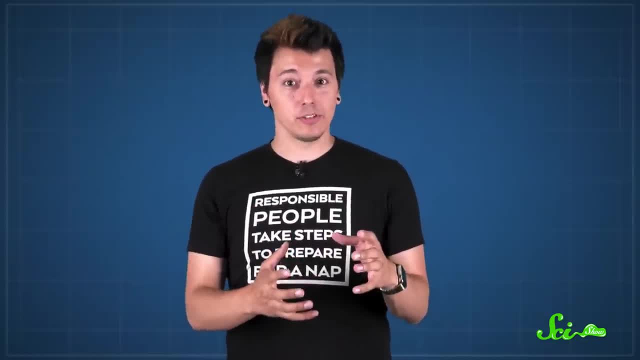 So it's possible that element 173 might actually be faster than the speed of light. It could actually be the end of the periodic table, Though we don't know for sure. Elements tend to be more and more unstable as they go up in number. 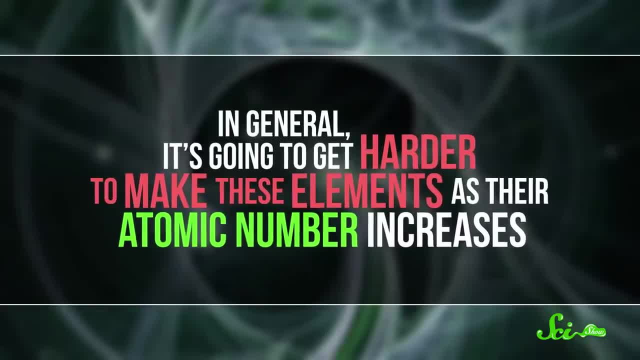 Which means that, in general, it's going to get harder and harder to make these elements as their atomic number increases. All the new elements we've been making recently only exist for the tiniest fraction of a second before they decay into smaller atoms. 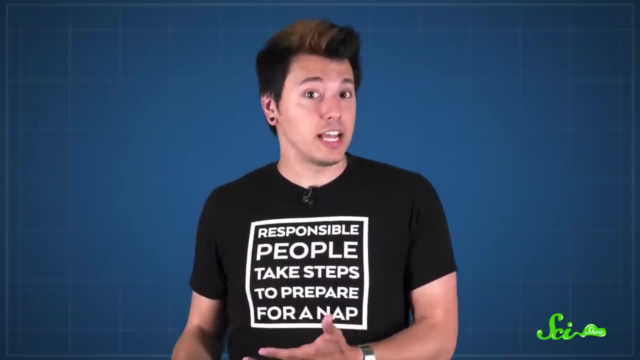 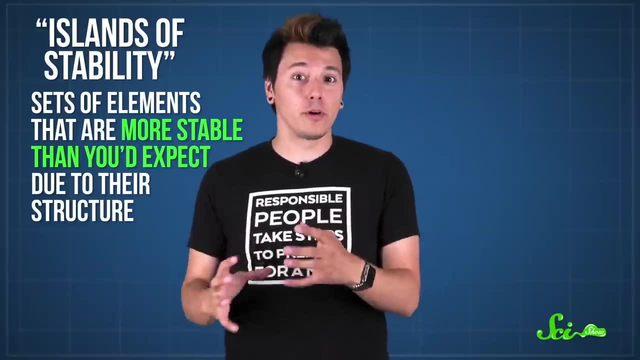 And maybe there's going to be some point when we just can't make them anymore because they're so unstable. But physicists have also predicted what are known as islands of stability, Sets of elements that are much more stable than you'd expect because of the way their protons and neutrons are organized in the nucleus. 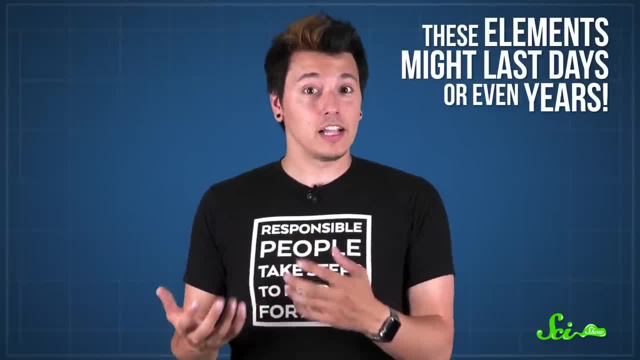 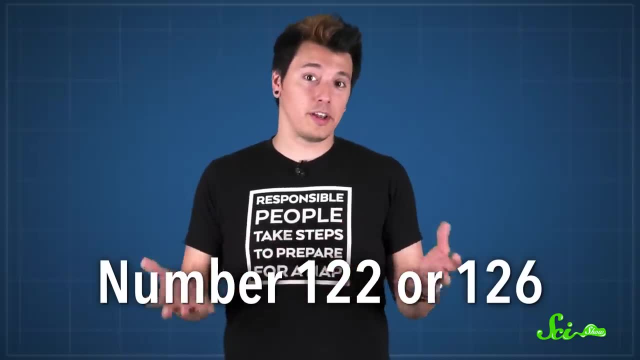 Instead of lasting only a tiny fraction of a second, these elements might last days or even years. Some predictions say that the first island of stability might start right around number 122 or 126, depending on who you ask and how they did the calculation. 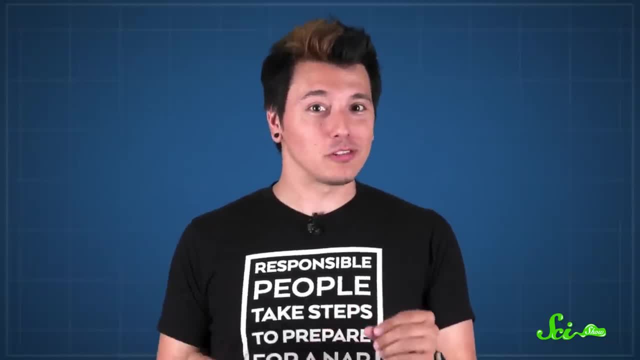 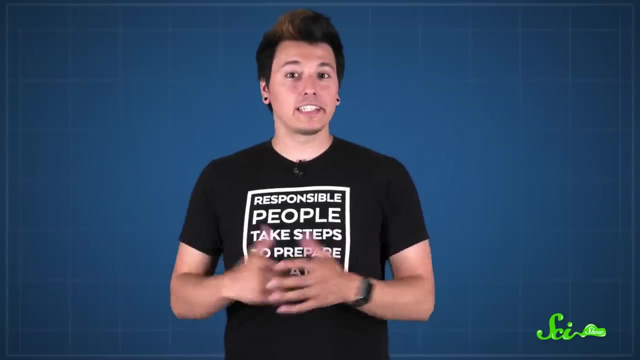 And since we've already made all the elements up to 118, we're pretty close, Which means that soon we might be learning a whole lot more about islands of stability and how big our periodic table can really get. Thanks for watching this episode of SciShow, which was brought to you by our patrons on Patreon, like Paul Garrett and Kelia Silvas. 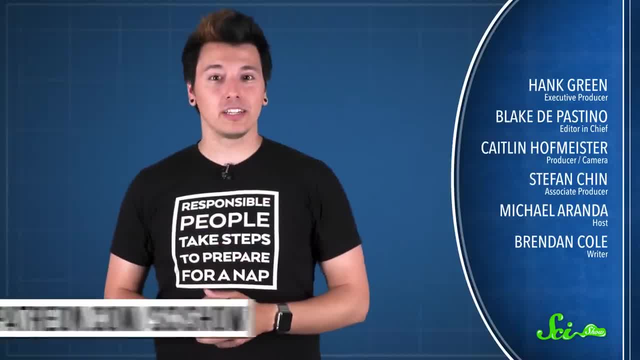 Thank you, Paul and Kelia. If you want to help support the show, you can go to patreoncom slash scishow. And don't forget to go to youtubecom slash scishow and subscribe.